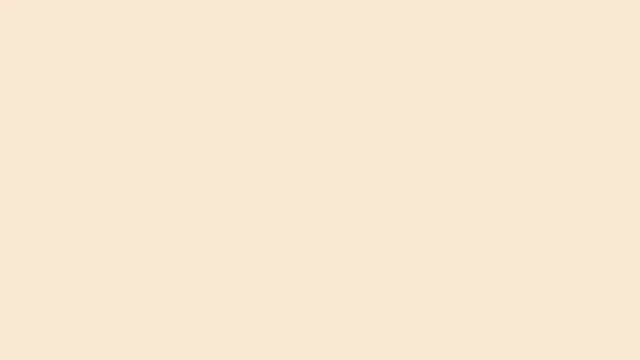 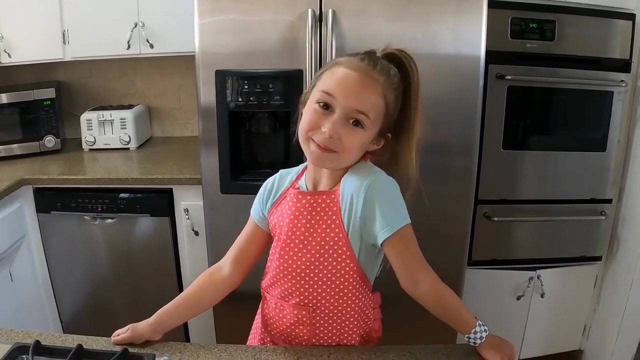 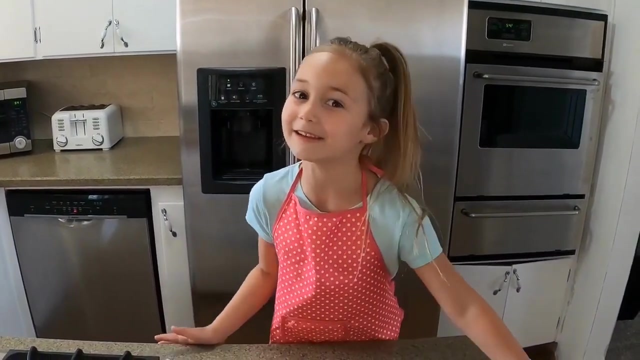 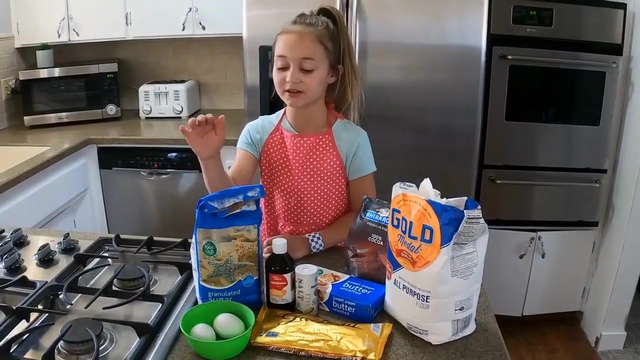 Welcome to Cooking with Taylee. Today we're going to make ooey gooey brownies. Before we get started, ask your parents to get the ingredients down below. Let's get started. Our ingredients for today are sugar, vanilla, salt, unsalted butter. 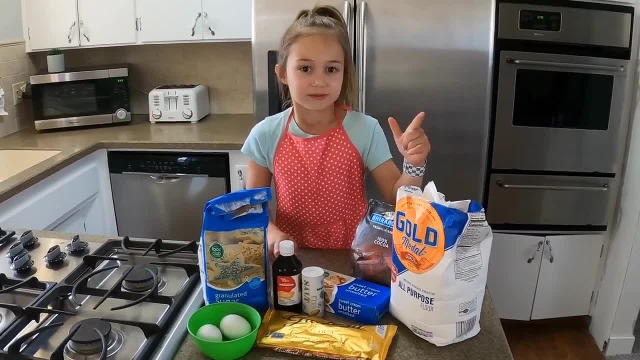 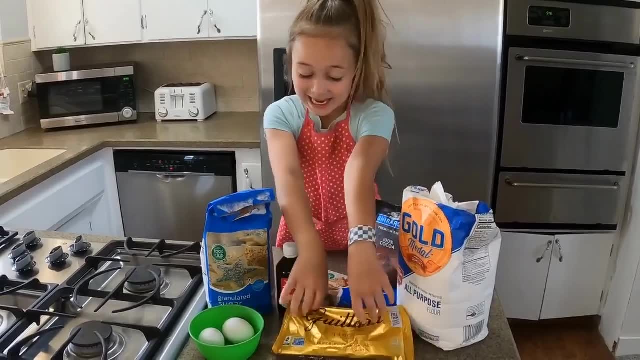 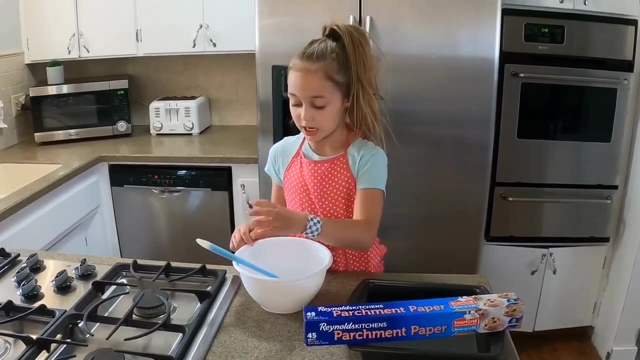 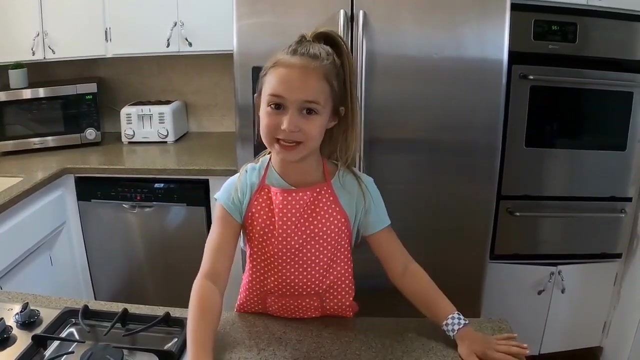 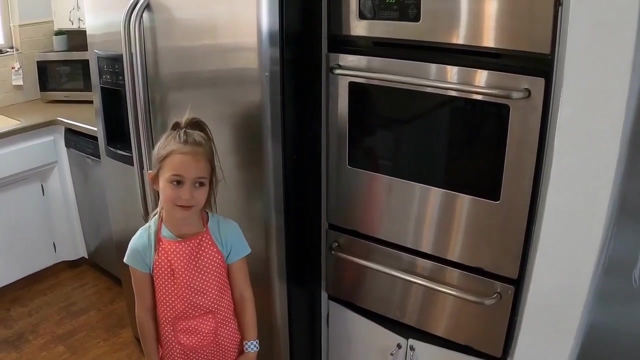 cocoa flour- big fat chocolate chips are my favorite- and two eggs. You're also going to need parchment paper, a pan, a bowl and a mixer. Now that you've got everything ready, let's get started. Ask your parents to put the oven to 350 degrees. 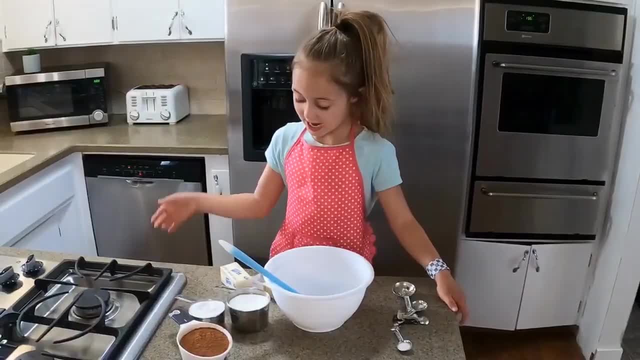 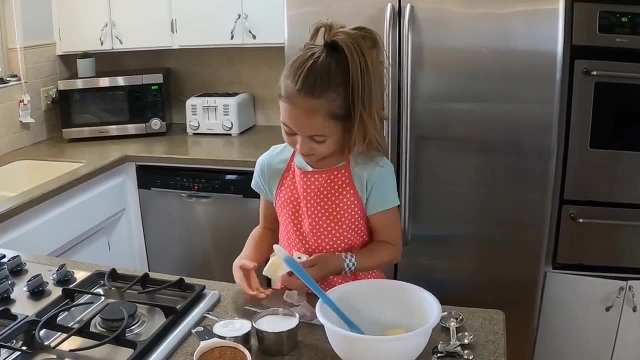 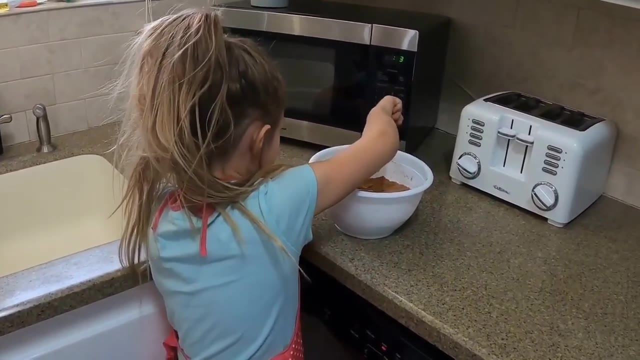 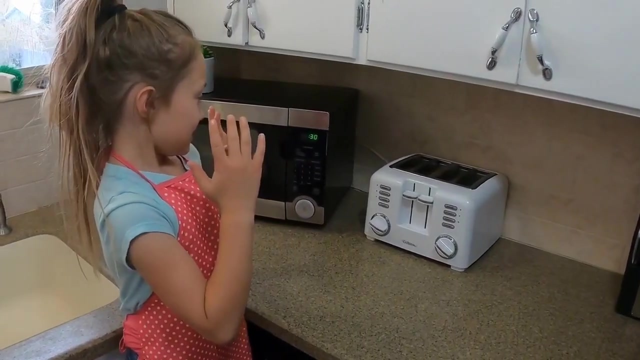 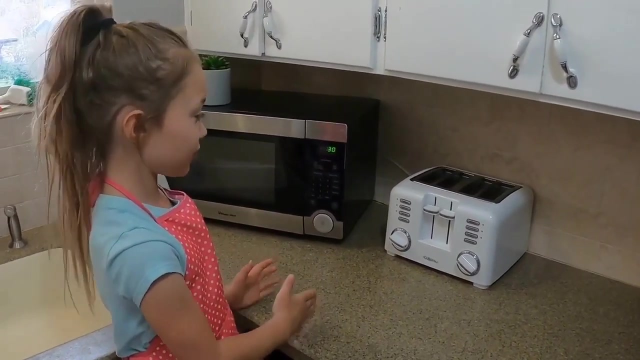 We're going to add the butter, the sugar, the cocoa and the salt. I'm going to be putting it for 30 seconds. We're going to put it in the microwave for 30 times until the butter is all melted. You limit 30 seconds at a time. 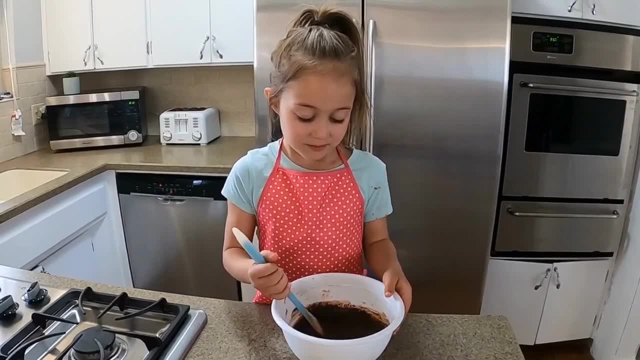 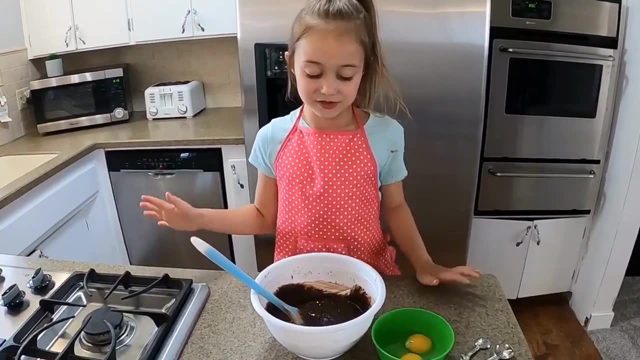 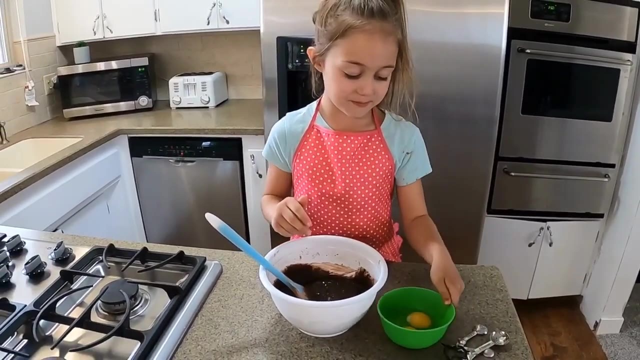 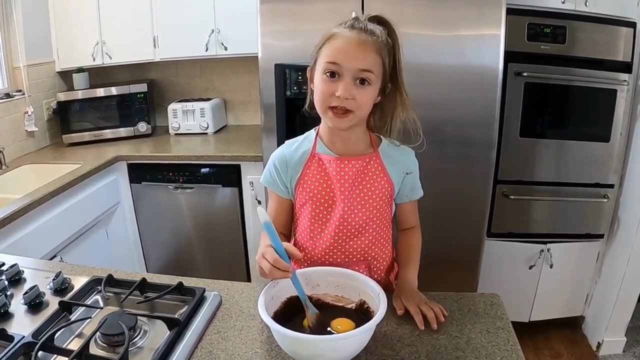 Now that the butter is melted, make sure to give it a good mix. After the butter is melted and you are done giving it a really good mix, you are going to add two eggs and some vanilla. After you are done with that, you are going to start mixing.